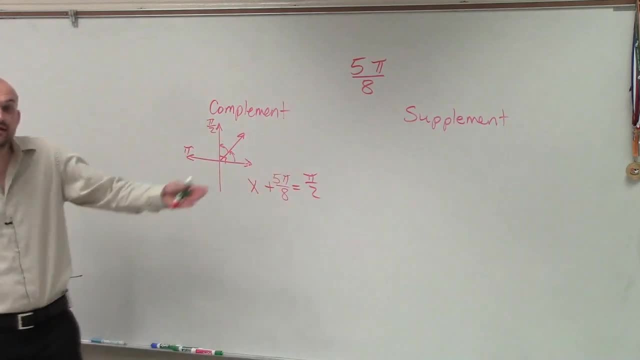 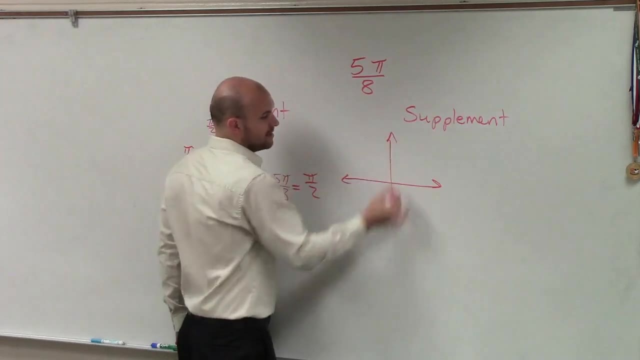 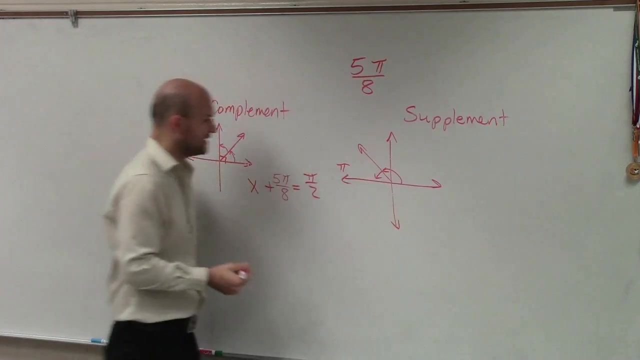 in there: 5 pi over 8.. Then what the supplement says is: find two angles that add up to give you 180 degrees, And remember, the radian measure of 180 degrees is pi. So we want to find two angles that add up to 180 degrees, But remember, since we're talking about radians, 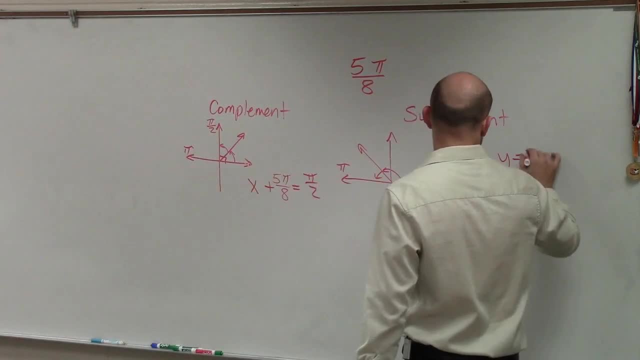 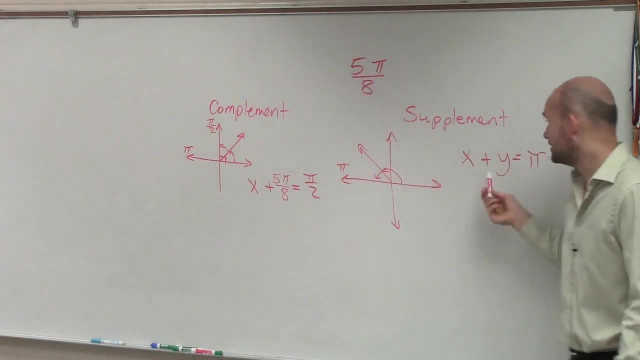 today or for this problem, it's going to be equal to pi. So when I say find the supplement of this angle, I'm saying what angle added to 5 pi over 8 gives you pi. And again we already know what the one angle is, which is 5 pi. 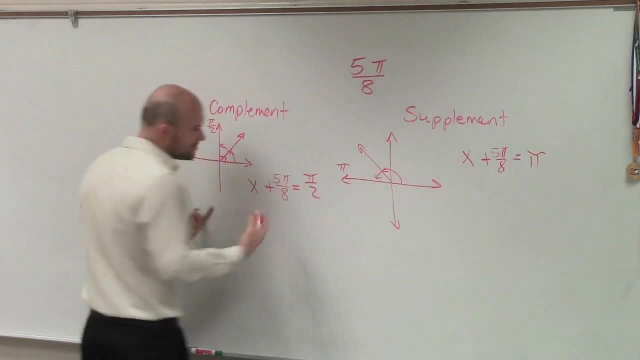 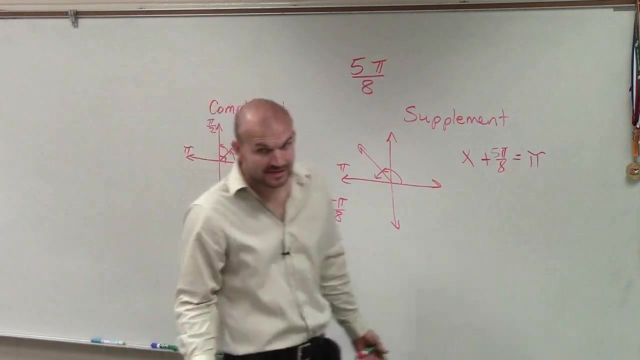 over 8.. So now, ladies and gentlemen, we just have an algebra problem. All we've got to do is now solve for x, So you subtract 5 pi over 8.. Subtract 5 pi over 8.. So there are x equals pi, halves, minus 5 pi over 8.. Now the problem comes in, though, is because 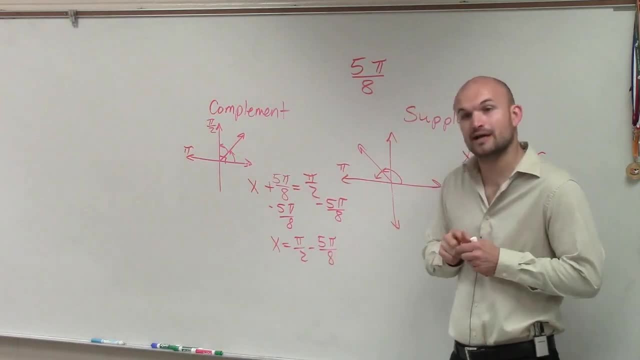 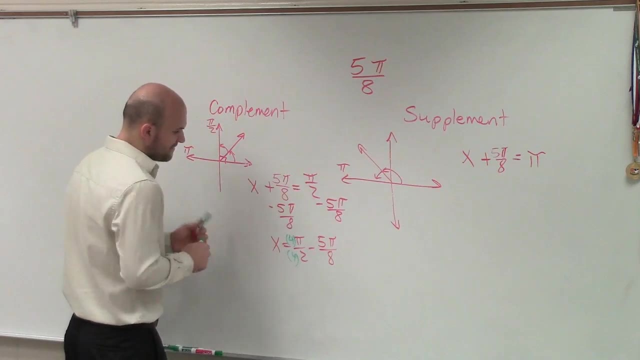 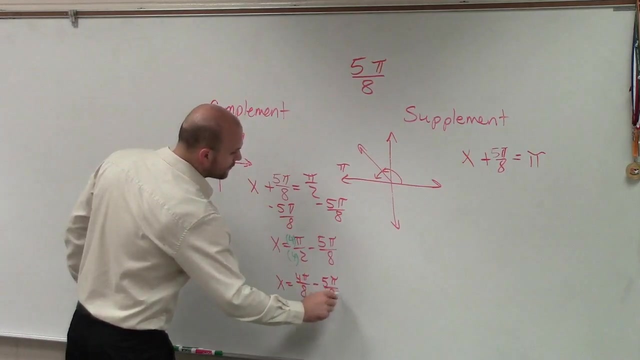 we don't have the same denominators, right? So therefore you've got to multiply by 4 over 4 to get like denominators. So my final answer: so I have x equals 4 pi over 8, minus 5 pi over 8, which equals a negative pi over 8.. Well, ladies and gentlemen, when we're 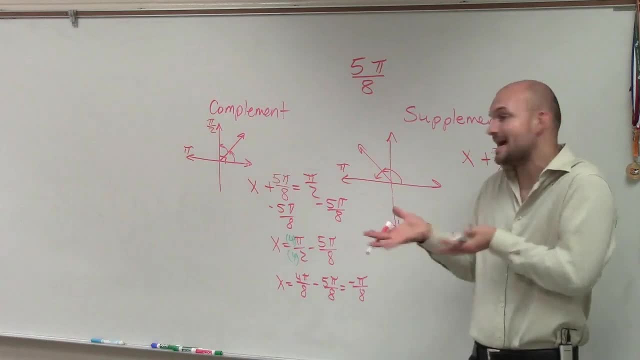 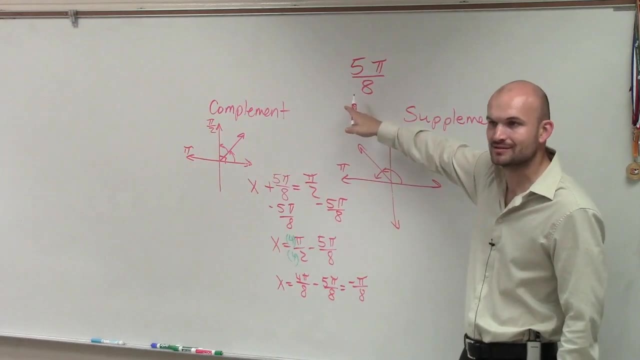 trying to find the complement. we're trying to find two positive angles that add up to pi halves. So if I have a negative angle, what that means is 5 pi over 8 minus 5 pi over 8 is already over 90 degrees. right, If you were to take, because 4 pi over 8 would. 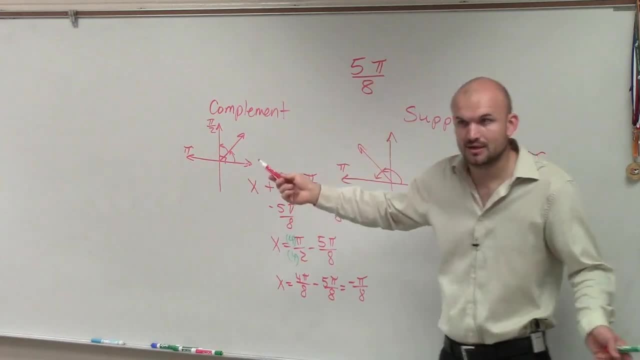 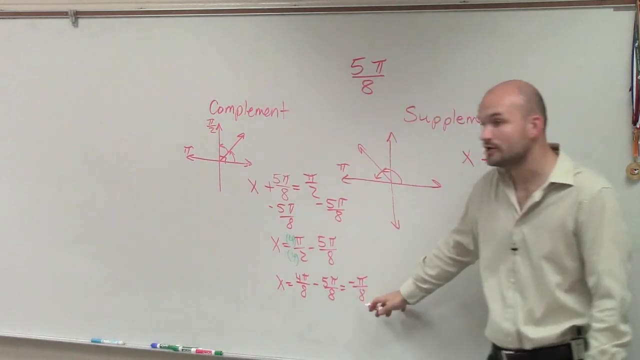 be pi halves. So 5 pi over 8 is over 90 degrees. So therefore this angle does not have a complement. okay, So you'd write. so, if you try to find the complement and you get a negative angle, it does not have a complement because it's already pi halves, It's already over 90 degrees. 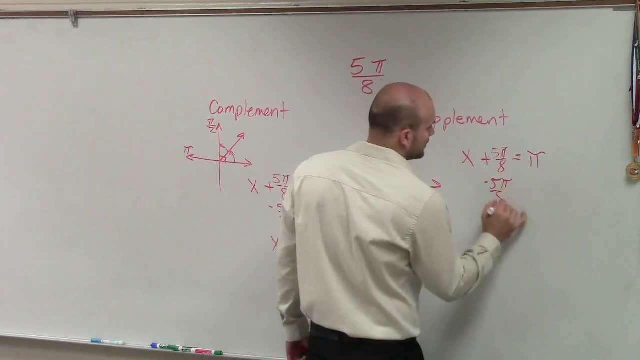 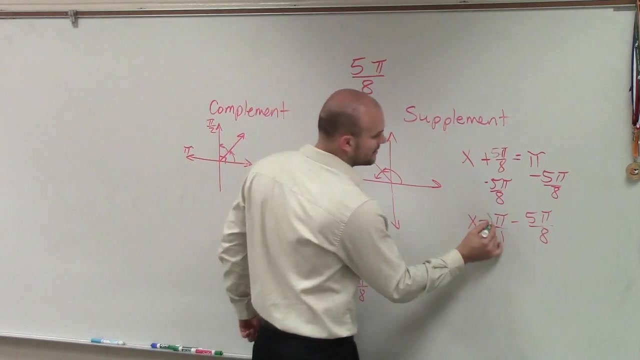 So let's go and do the supplement. So I subtract 5 pi over 8.. So therefore I have x equals pi, minus 5 pi over 8.. Again, we need to get the common denominator, so I'll put this over 1. And then multiply. my voice is like dying multiply. 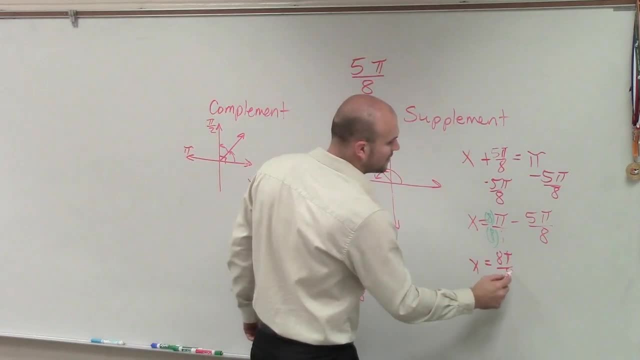 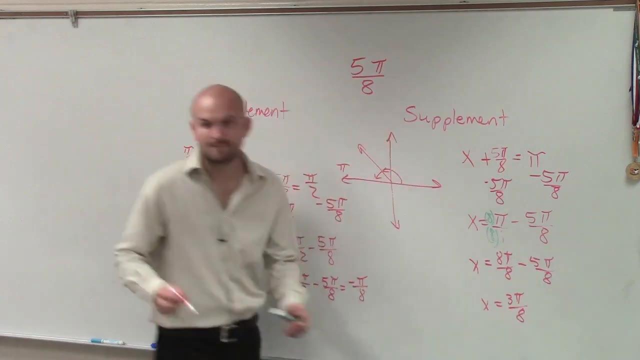 by 8.. So now I have x equals 8 pi over 8, minus 5 pi over 8. So x equals 3 pi over 8. Cool, So the complement does not exist, but we have a supplement of 3 pi over 8.. I will. 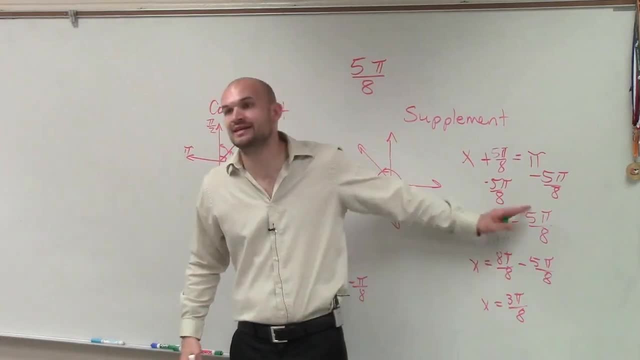 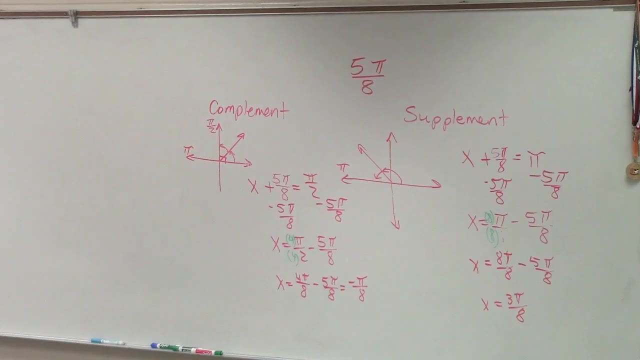 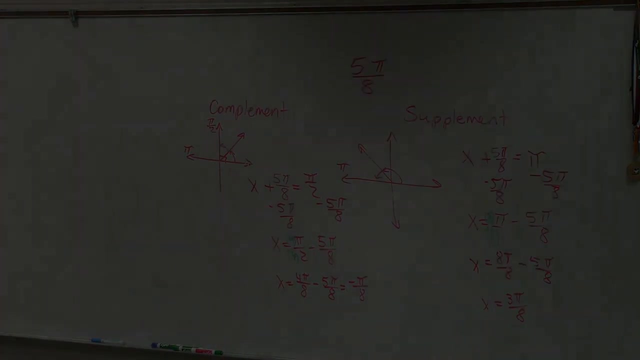 tell you guys, right now we are going to be doing a lot of getting the common denominator, adding and subtracting your fractions. This will become very, very important. I probably should have given you guys a worksheet extra on doing these, for Will. 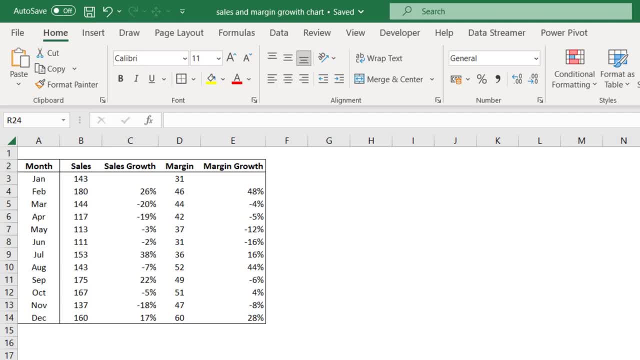 I have the sales and margin data of a company for 12 months and I want to create charts to plot these four parameters. The parameters are sales, sales growth percentage, margin and margin growth percentage. I'm actually going to put these charts on a dashboard. 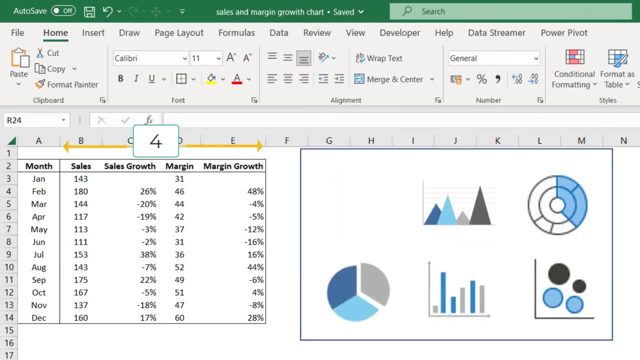 But the problem is that my dashboard already contains several charts. There is not much space left and I can add only one more chart to the dashboard. So I need to plot all these four parameters on a single chart and I want to make sure that the chart still looks good. 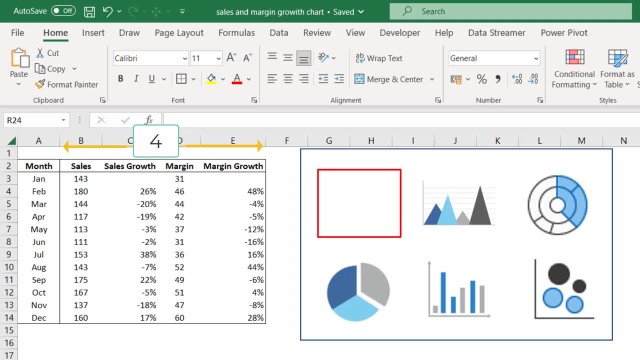 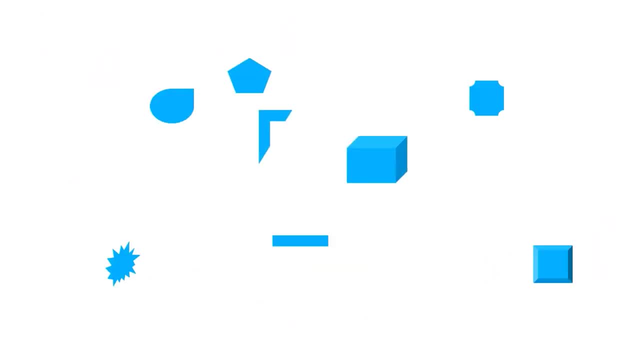 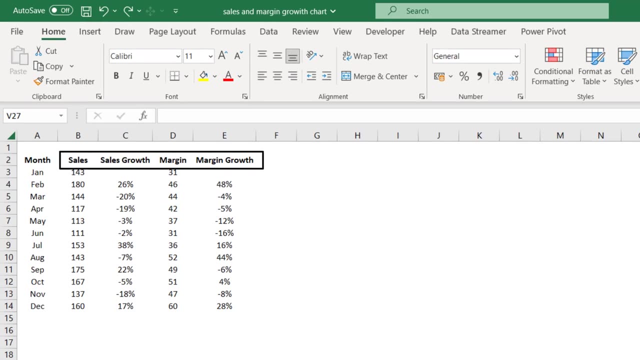 does not get cluttered and is easy to read. So let's see how can we create the best chart that we are looking for. So this is our data and we want to plot these four parameters on a single chart. We're going to create a combo chart of column charts and line charts- Two of our parameters: single. 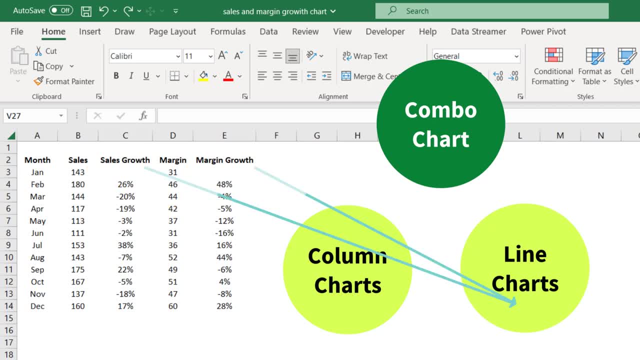 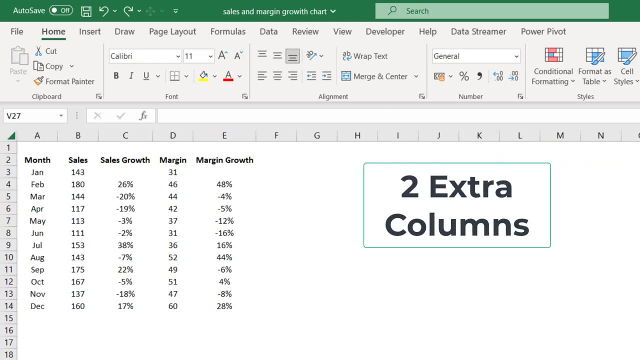 sales and margin will come on columns and the other two will come on line. So let's create this interesting chart, But before that we need to insert two additional columns in our data. These columns will only help us to create the chart, So let's insert a.